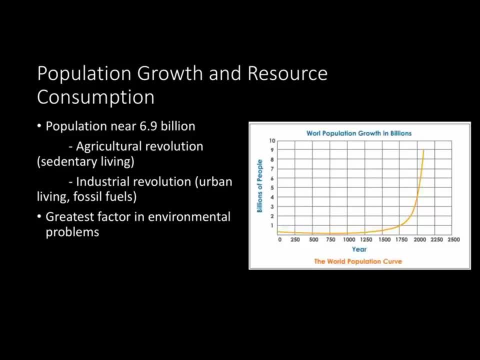 Population growth and resource consumption. Currently, the population of the world is somewhere near the 6.9 billion mark. In environmental science, there are two important times in population trends to really look at. First, the agricultural revolution. So essentially, the agricultural revolution was when people ceased to be nomadic and instead. 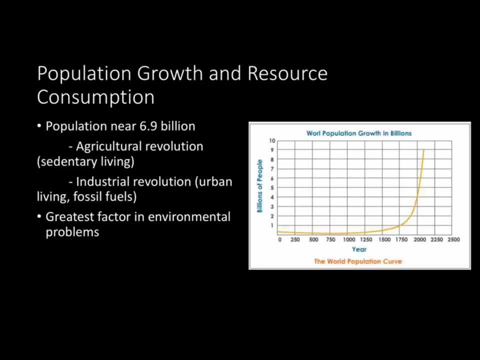 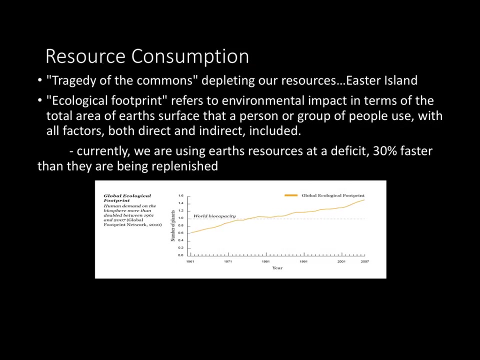 settled down in one place and started farming. Another important area to look at is the industrial revolution, which is when people left those agricultural centers and moved to urban centers where they started manufacturing and burning fossil fuels. Population is the single greatest factor in environmental issues. Resource consumption: A main topic in environmental 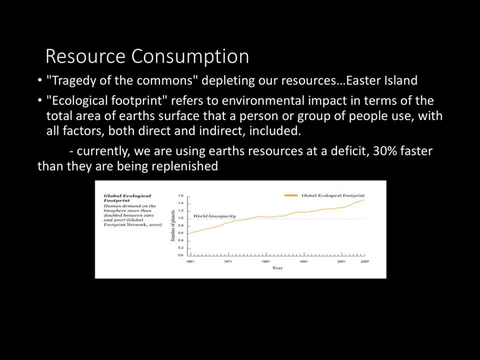 science is something known as tragedy of the commons. Tragedy of the commons basically means that a common source that no one really owns is being depleted, and since nobody owns it, no one really takes care of it. A prime example of this comes from Easter Island, which is 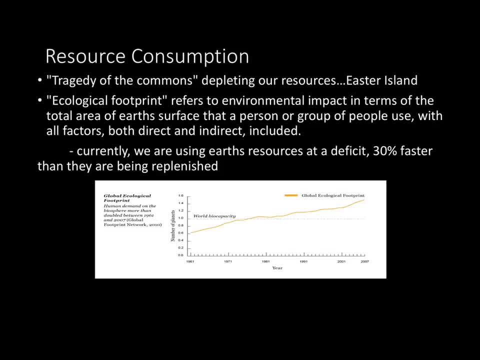 exemplified in the book On Easter Island. it was a thriving population, but then at one point, they decided to cut down all their trees. Right after they cut down all the trees, the population dipped down and the entire civilization collapsed. Another important topic is an ecological 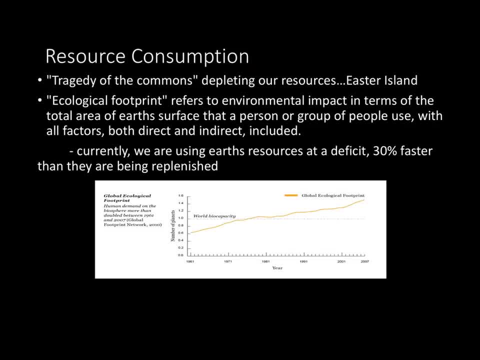 footprint. This basically refers to an environmental impact in terms of the total area of earth's surface that a person or group of people use, with all factors, both direct and indirect, included, If you refer to the graphic down here. currently we are using 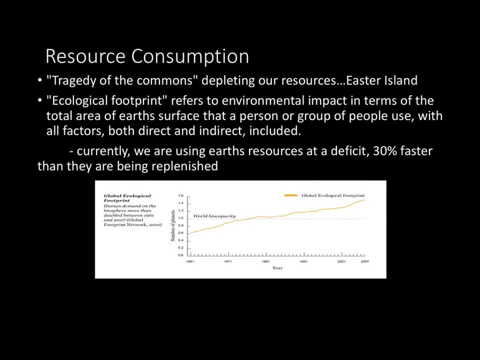 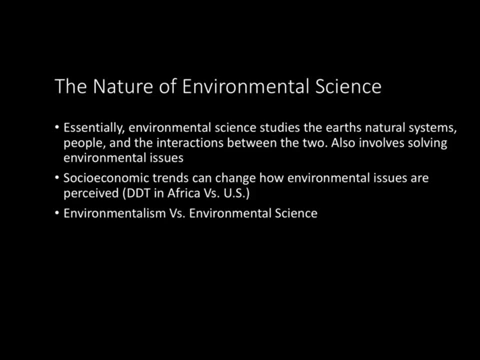 the earth's resources at a deficit of 30% faster than they are being replenished. The nature of environmental science: Essentially, environmental science studies the earth's natural systems, people and the interactions between the two. This also involves solving environmental issues. How someone values an environmental issue can really depend on socioeconomic trends. 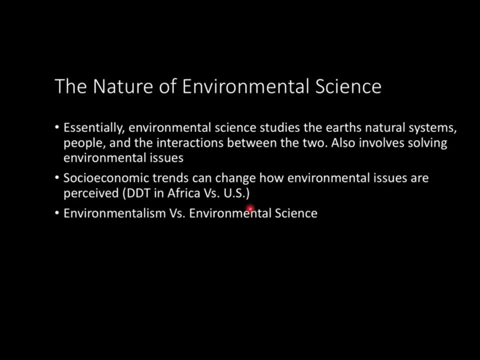 as discussed in your book, with the difference between DDT in Africa and DDT in the United States. An important differentiation to make is between environmentalism and environmental science. Environmentalism is a social issue bent strictly on defending the natural world, while environmental science is essentially a study of the interactions between humans. 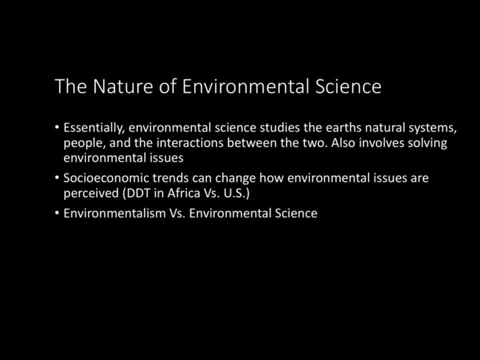 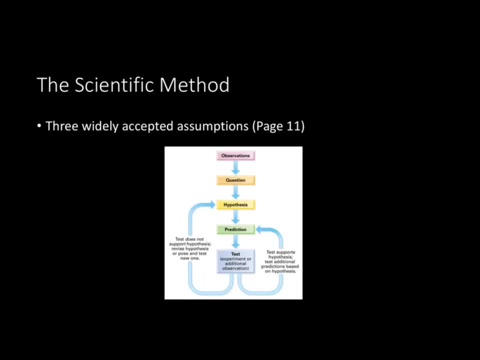 the environment and solutions to solve problems between the two, The scientific method. So if you refer to page 11, there are basically three main aspects of the scientific method that are widely accepted. First off, The universe functions in accordance with the fixed natural laws. 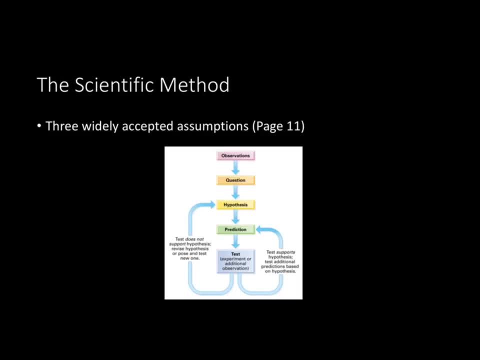 that do not change from time to time or from place to place. Next, all events arise from some cause or causes and in return cause other events. And third, we can use our senses and reasoning abilities to detect and describe natural processes that underlie the cause and effect relationships we observe in nature. 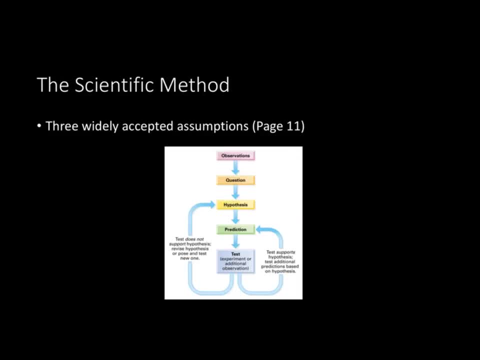 Also, the model of the scientific method is also widely accepted. It basically reads: observation leads to questions, to a hypothesis, to a prediction, to a test, to results and then, based on those results, you could look and reinterpret your prediction. 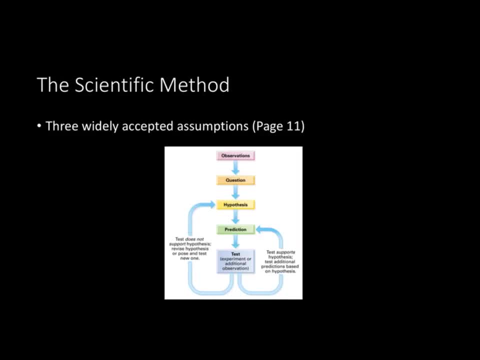 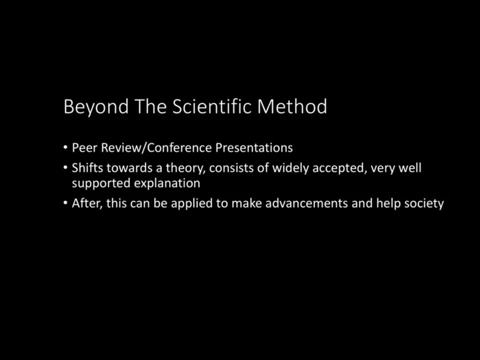 and you can look back and reinterpret your hypothesis Beyond the scientific method. Essentially, the scientific method continues to include a few more main areas. In the peer review process, scientists give their work to another group of scientists to evaluate the quality. They also present the work at conferences. 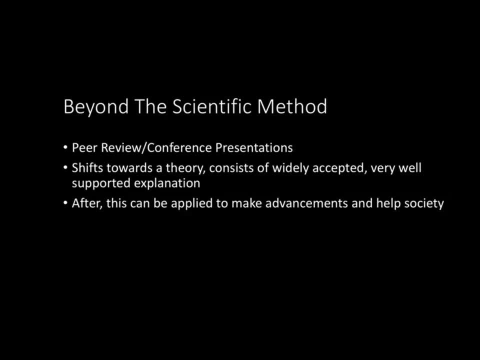 in order to gain feedback. Eventually, if validated, the work could mold into a theory which is a widely accepted, very well-supported explanation of an issue. From here, said work could be applied to make advancements that we could use in our modern society. 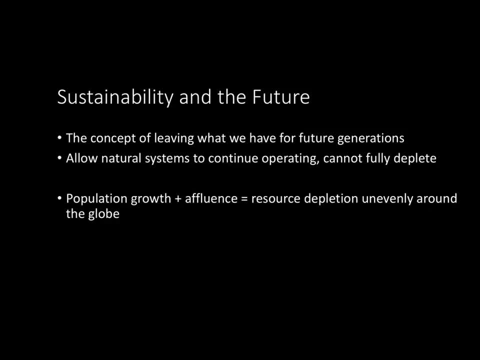 Sustainability and the future. Sustainability is basically the concept that we should leave the same world for future generations, But in order to do this, we cannot fully deplete the natural world Together. population growth and affluence are the main source of modern resource depletion. 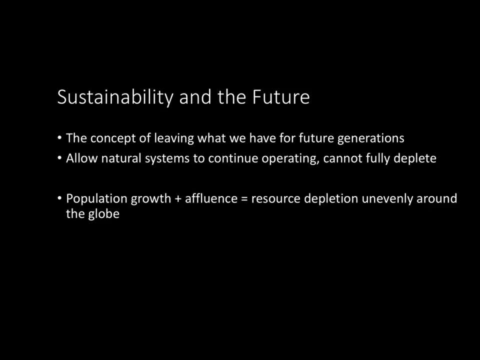 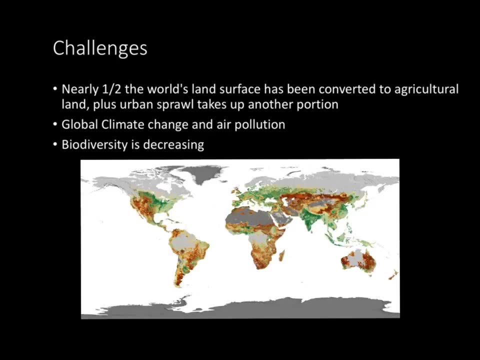 and this happens unevenly around the globe Challenges. Currently, nearly one half of the world's land surface has been converted to agriculture, Plus urban sprawl takes up another large portion of this: Global climate change and air pollution. Global climate change is another huge issue in environmental science. 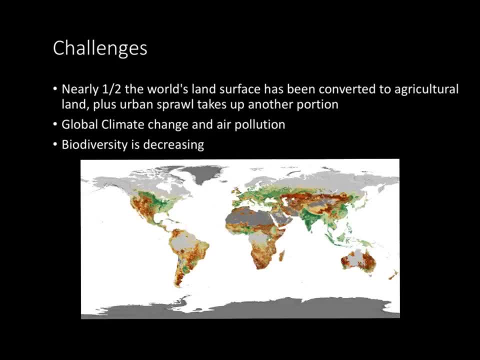 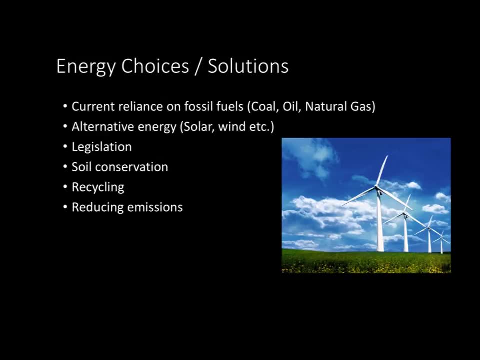 and its effects are leading to a decrease in biodiversity, And when biodiversity is decreasing, this shows an uneven, unstable environment, Energy choices and solutions. Currently, we rely heavily on non-renewable resources such as fossil fuels, which not only hurt the environment,